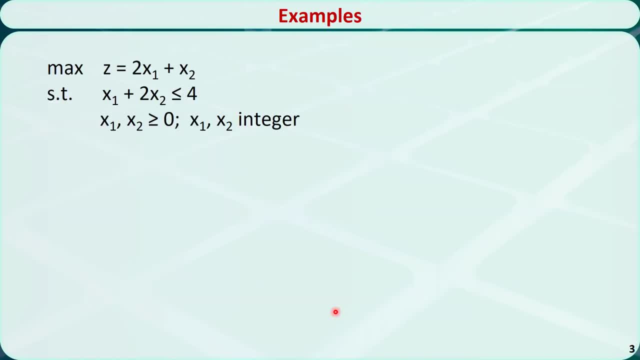 Thank you for watching. Let's check some examples. This is a maximization problem with two decision variables: x1 and x2.. They are both required to be greater than or equal to 0, and they are both required to be integer numbers, so it is a pure integer programming problem. This is the second example. 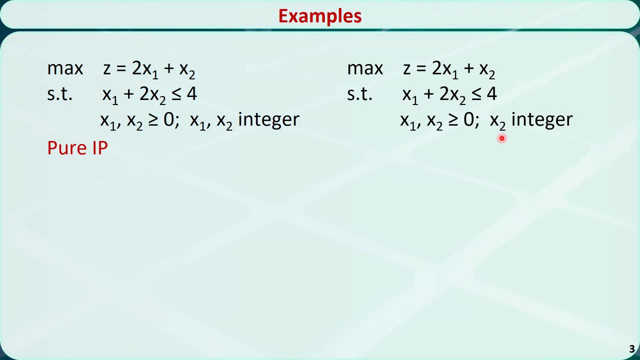 The only difference is that only x2 is required to be an integer and x1 is not required to be an integer, So it is a mixed integer programming problem. This is the third example. The difference between this one and the first one is that 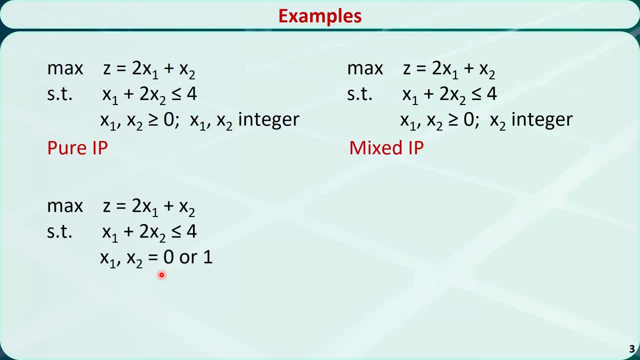 both x1 and x2 are required to be binary. That means either 0 or 1.. So it is a 0-1 integer programming problem. This is the last example. The only difference between this one and the first one is that. 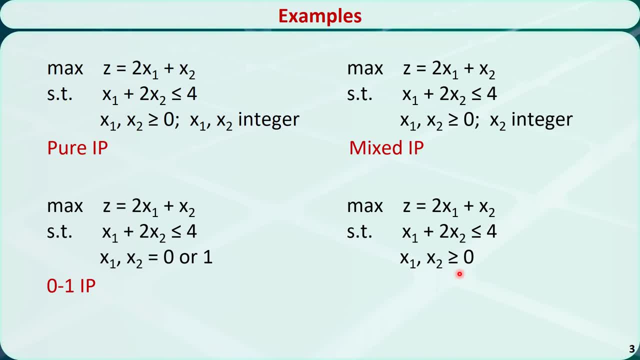 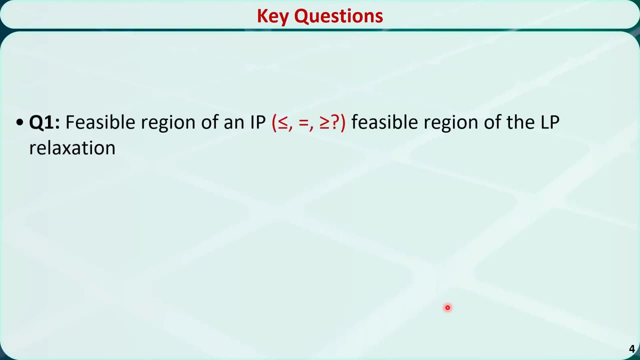 there is not an integer requirement for the decision washing. In a business model solution, the decision variables. This is a linear programming problem because both the objective function and the constraint are linear. It is called the linear programming relaxation of the first three examples. Now let's answer four questions. 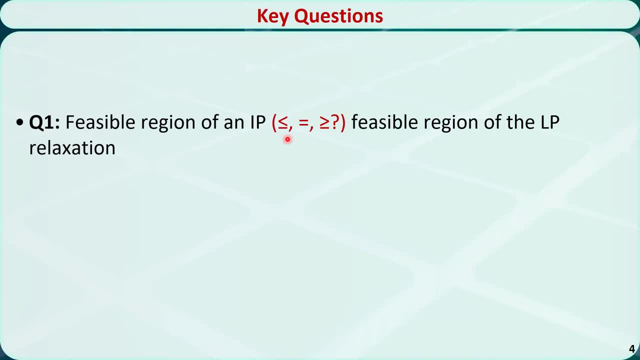 Question 1.. Which problem's feasible region is larger, an integer programming problem or its linear programming relaxation? The answer is that, in general, the linear programming relaxation has a larger feasible region. This is because the variables can take both integer numbers and fractional numbers in the linear programming relaxation. 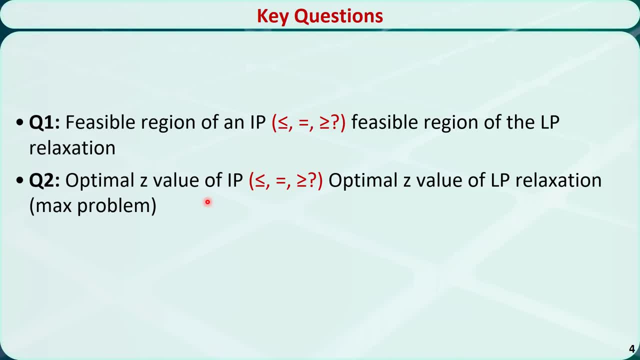 Question 2. For a maximization problem, which optimal z value is larger, an integer programming problem or its linear programming relaxation? The answer is that, in general, the linear programming relaxation has a larger optimal z value. This is because the feasible region 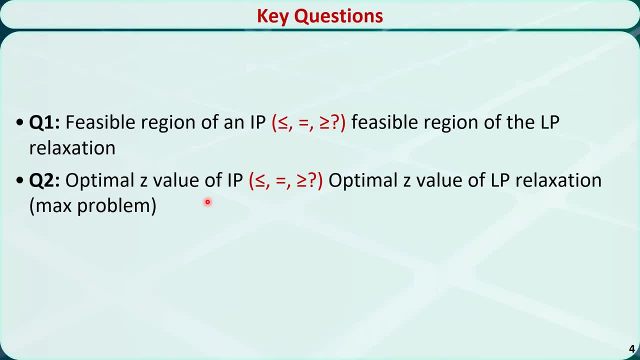 is larger for the linear programming relaxation and it has more options or a better chance to contain the largest z value. Similarly, for a minimization problem, in general, the linear programming relaxation has a smaller optimal z value. This is because the feasible 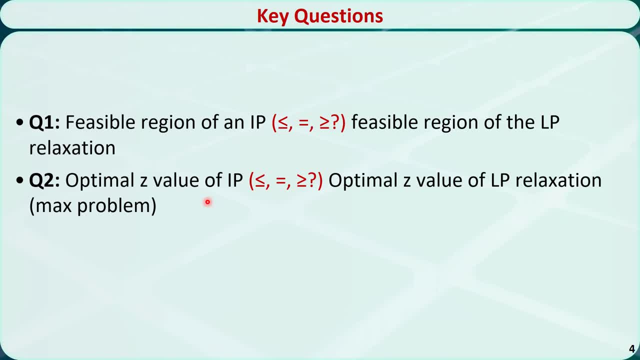 region is larger for the linear programming relaxation and it has more options or a better chance to contain the smallest z value. Question 3. Which one of the following is more difficult to solve: an integer programming problem or its linear programming relaxation? The answer is that, in general, an integer programming problem is more difficult to solve. 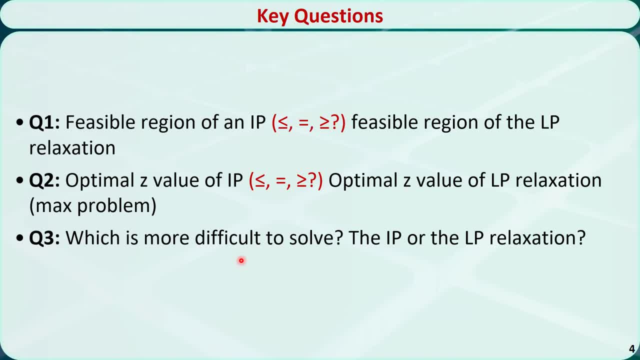 than the linear programming relaxation. This is because we can use the simplex method to check only the extreme points for the linear programming relaxation and there will be a path that leads us to the optimal solution For the integer programming problem. theoretically, we need to enumerate all the possible integer combinations in the feasible region and check. 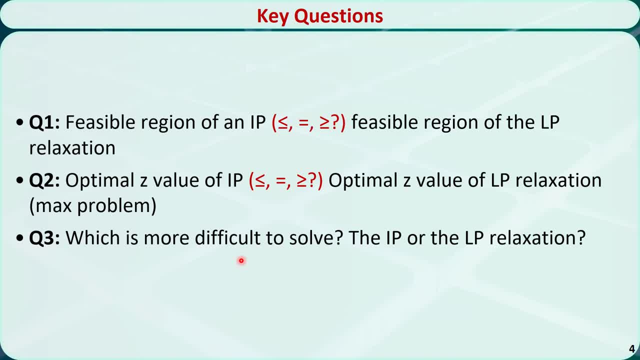 their z values before we can conclude which one or which ones are the optimal solutions. Question 4. Can we use the rounding method to solve an integer programming problem? That means, after we get the optimal solution for the decision variables to the linear programming relaxation, can we round these variables to the nearest integer and claim that the rounded 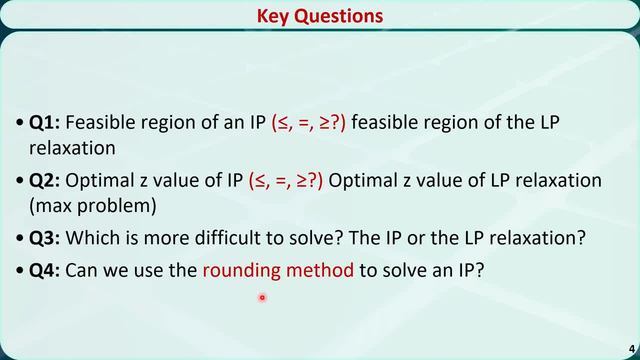 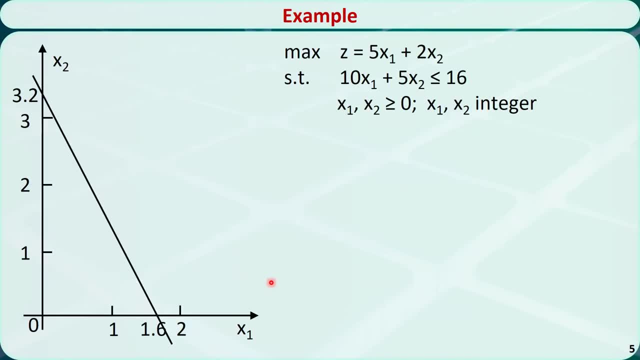 solution is the optimal solution? The answer is no. Let's see an example. This is an integer programming problem with two variables, x1 and x2.. We can represent it in this figure. This is the constraint: Because x1 and x2 are both integer numbers, the feasible region contains just 6 points. 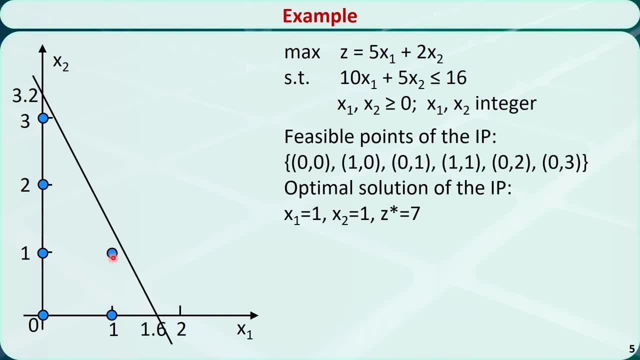 00,, 10,, 01, 11,, 02, 03.. We can check the z value of each point. The optimal solution is: x1 is equal to 1,. x2 is equal to 1, z star is equal to 7.. The feasible region of the linear programming: 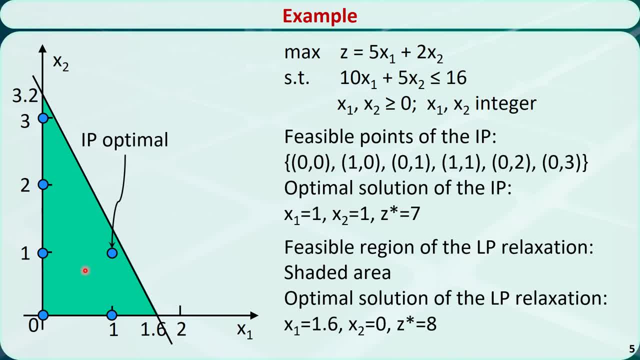 relaxation is marked by the shaded area. The optimal solution is this: extreme point: x1 is equal to 1.6. The optimal solution is this extreme point: x1 is equal to 1.6.. The optimal solution is this: extreme point: x2 is equal to 0, and z star is equal to 8.. If we round down to